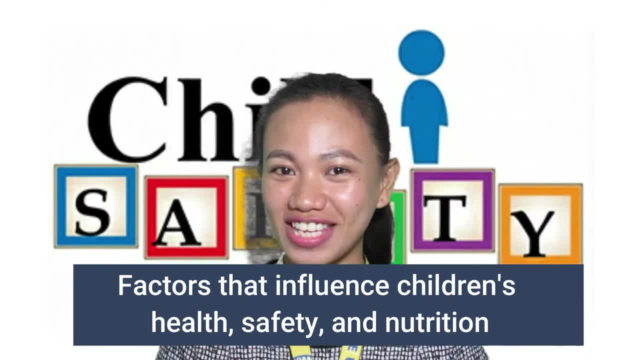 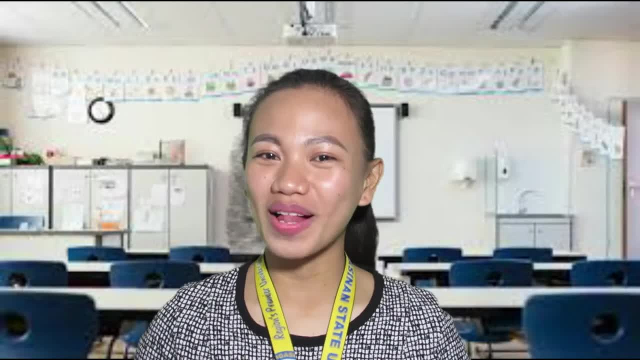 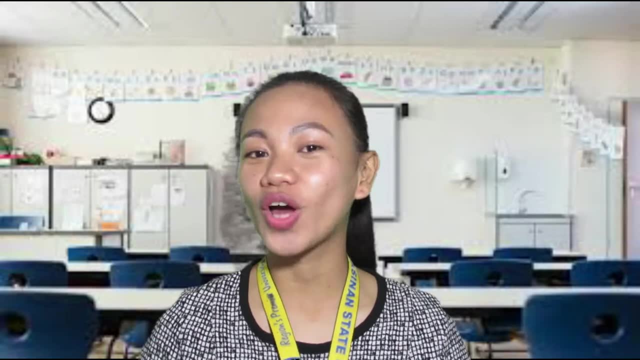 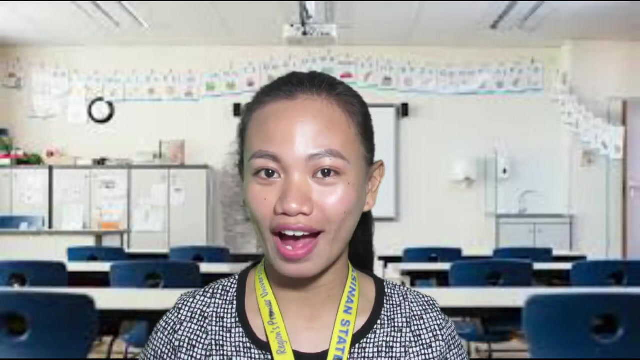 Factors that influence children's health, safety and nutrition. Hey guys, welcome back to my channel. This is me again, Teacher Pulene, And today I will be answering the question: What contributes to a child's overall well-being? There are four factors that affect child well-being. 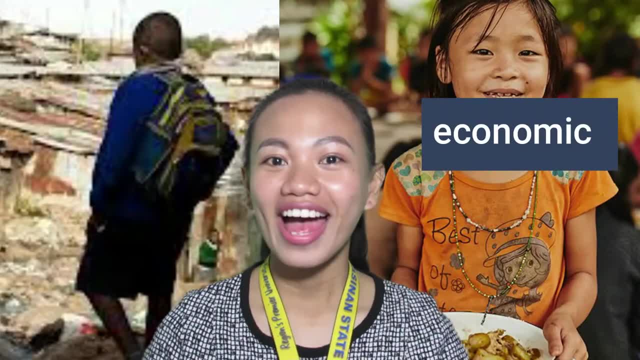 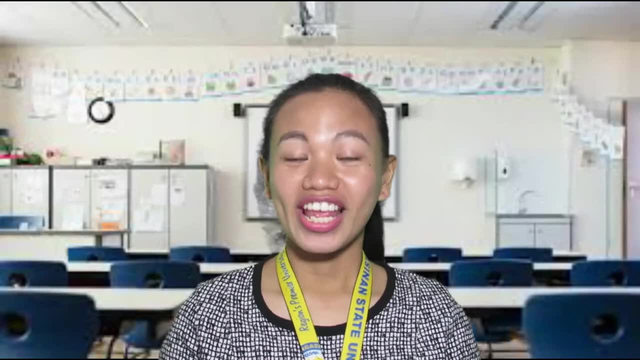 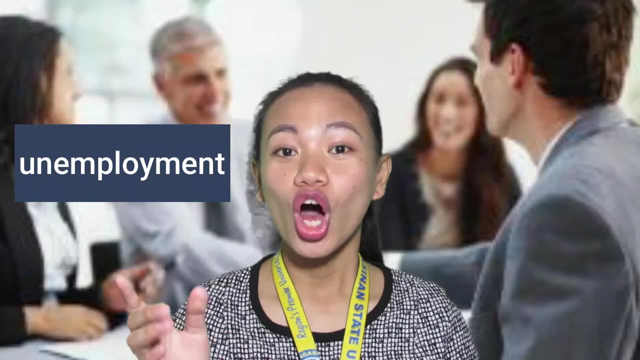 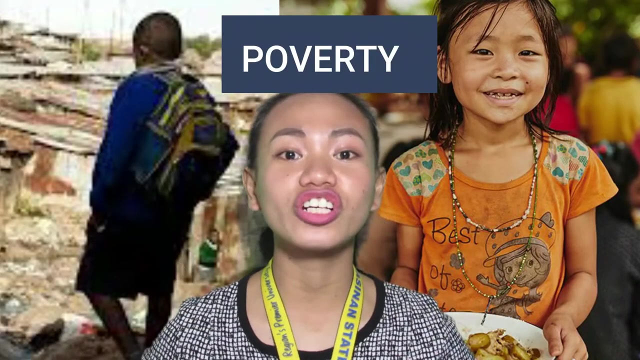 These are the economic, education, health and family and community factors. Let's begin with economic well-being factor. Including affordable houses and unemployment contribute to how parents can support their children. Growing up in poverty increases the risk of a child experiencing negative impacts. 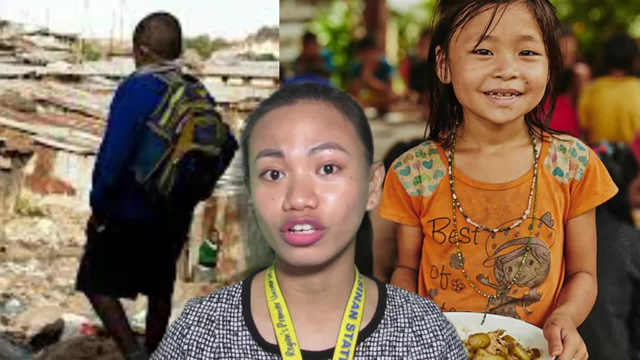 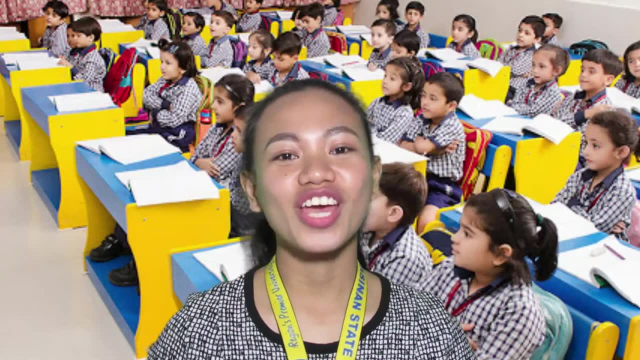 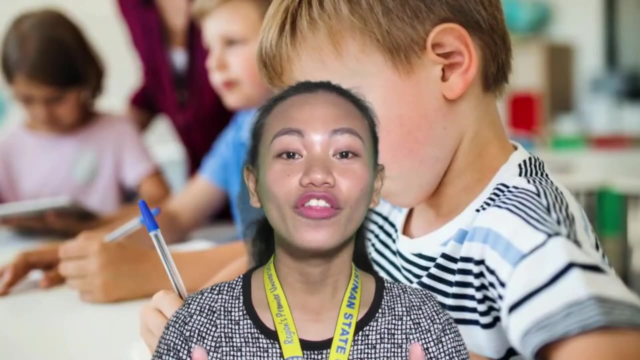 to their brain, Negative brain development, negative health outcomes and poor performance in school. Next is the education factors. Education factors can play a large role in a child's overall well-being and can affect their post-secondary plans which college they attend. 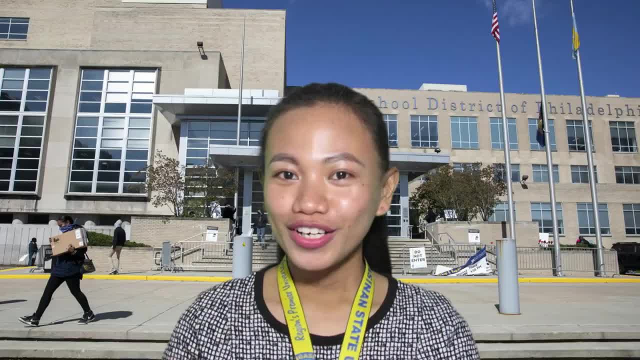 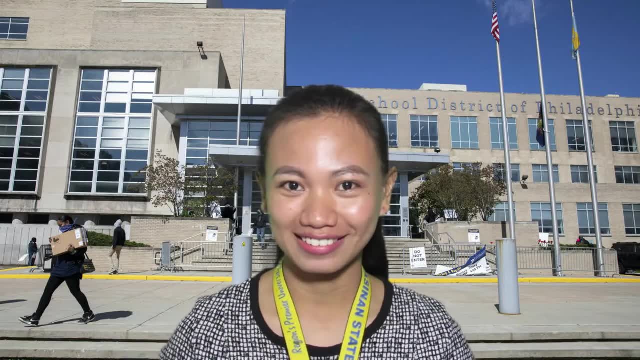 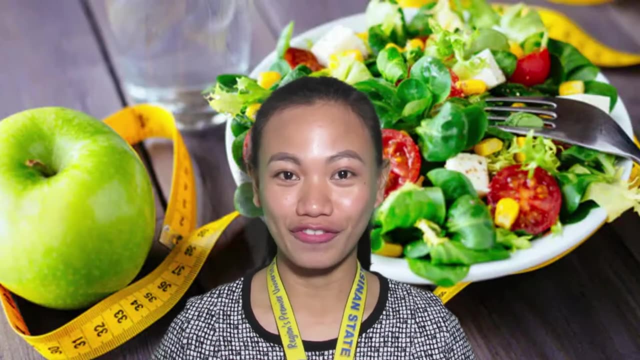 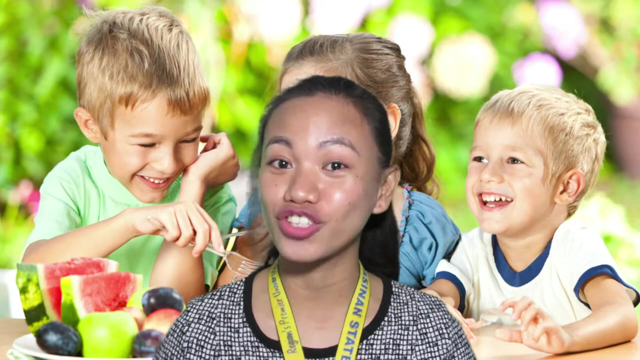 and what jobs they get as adults. Early in a child's life is a critical time to set a foundation for successful learning. Next is the health factors. Health factors add to the overall development of a child. Nutrition and access to good health care are both keys to ensuring a child is healthy. 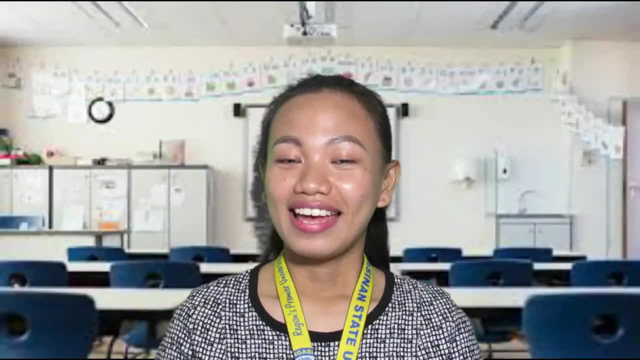 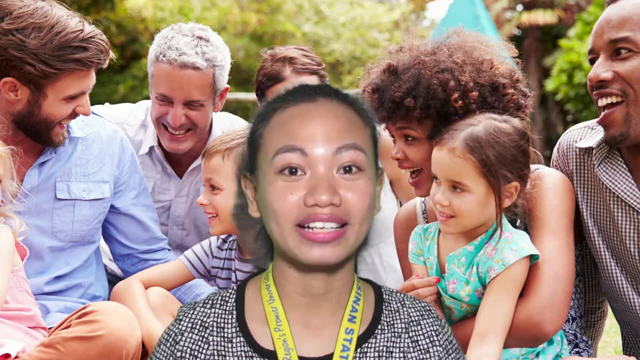 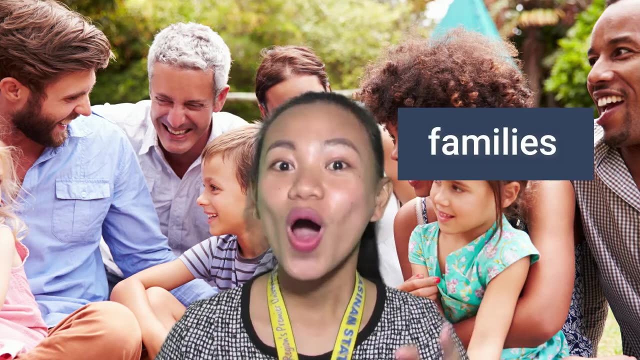 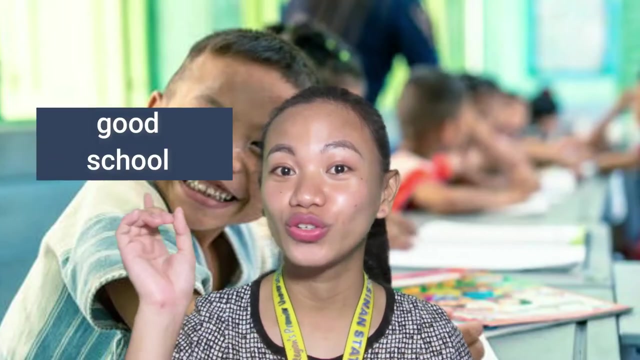 and can become a healthy adult. And lastly, family and community factors. Family and community factors impact children in unimportant ways. We know that children grow best in families with supportive and trusting relationships. to help them learn and grow, Children also need good school and good services to succeed. 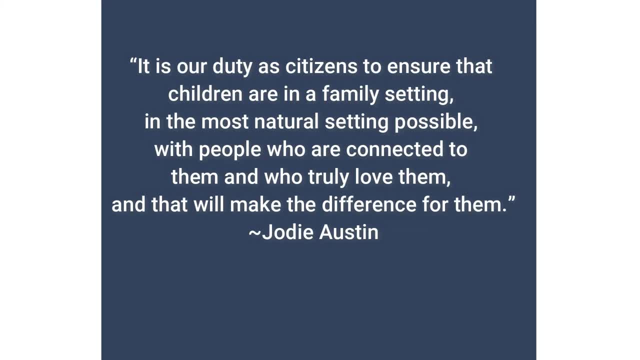 Jodi Austin said, It is their duty as citizens to ensure that children are in a family setting, in the most natural setting possible, with people who are connected to them and who truly love them, and that will make the difference for them. most people know that children need shelter.